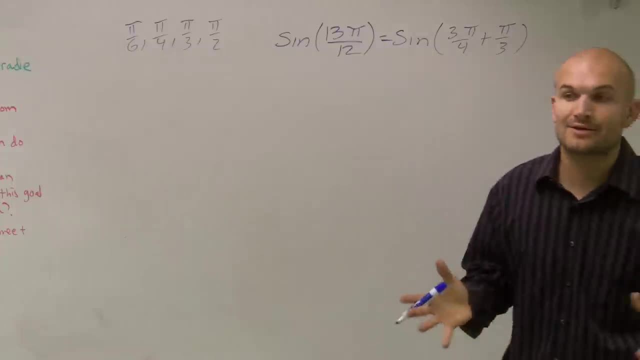 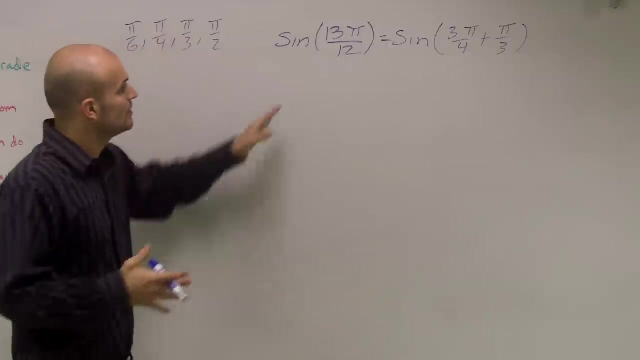 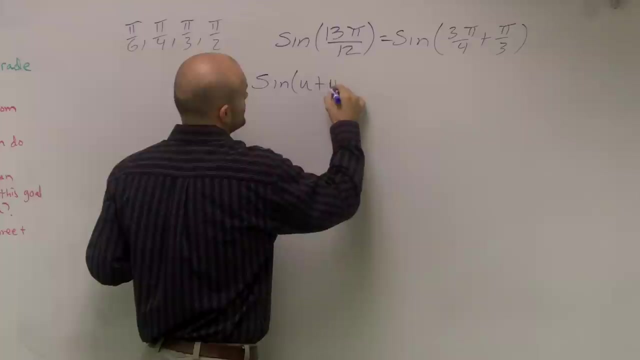 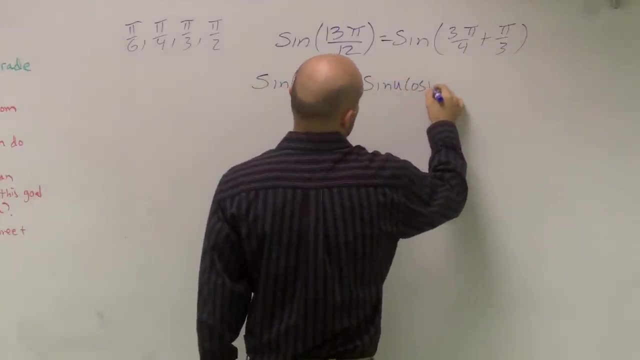 important, because now what I have is I have the sum of two different angles. So to solve for sine I can use the sum, The sum angle formula, for sine, And what that's going to look like is, if I have two angles, that I'm adding sine of u times, sine of v, what that equals is the sine of u times the cosine of v. 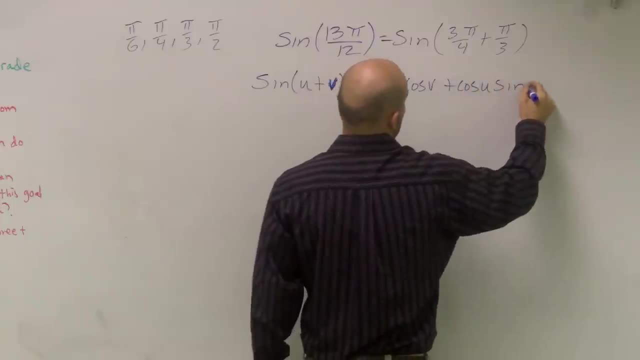 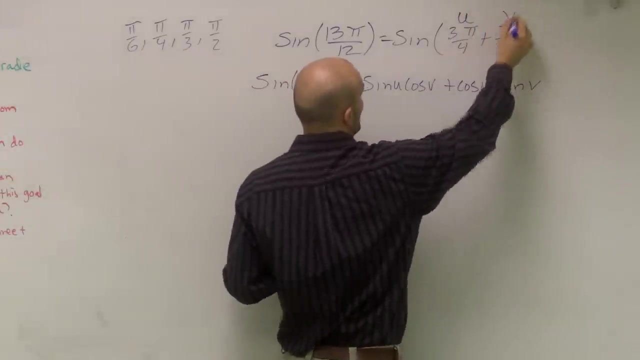 plus the cosine of u times the sine of v. So what I'm going to do is I'm going to let 3, pi over 4 be my u and pi over 3 be my v. So now I'm going to do this. 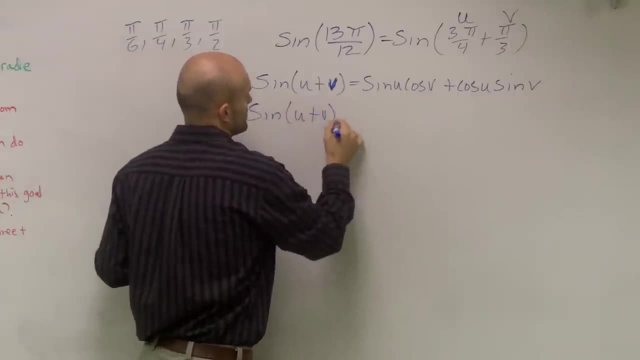 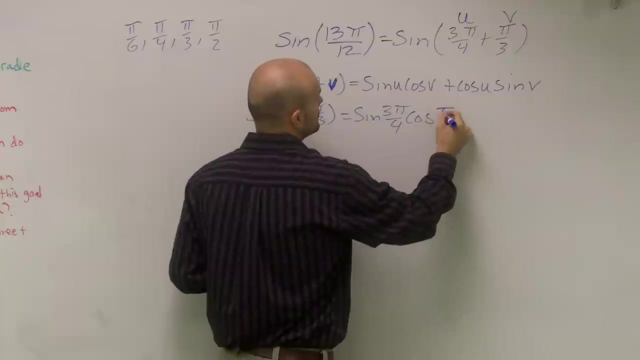 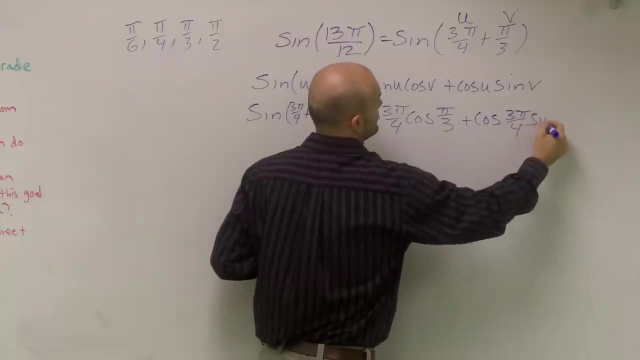 I'll write: sine of u plus v equals- I'm sorry- sine of 3 pi over 4 plus pi over 3 equals the sine of u, which is 3 pi over 4, times the cosine of pi over 3, plus cosine of 3 pi over 4 times the. 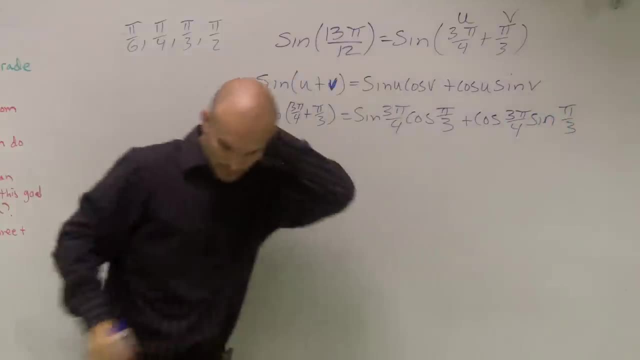 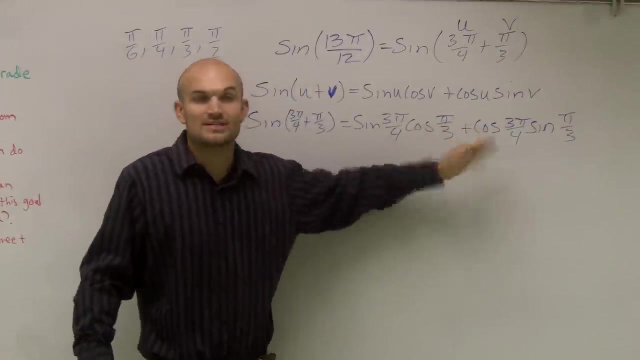 sine of pi over 3.. So now what I need to do is I need to determine what these values are. Now. luckily, these are all values that we know are on the unit circle, because I used multiples of these angles, So I can. 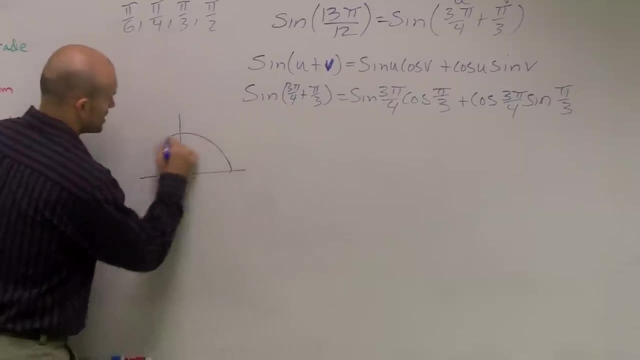 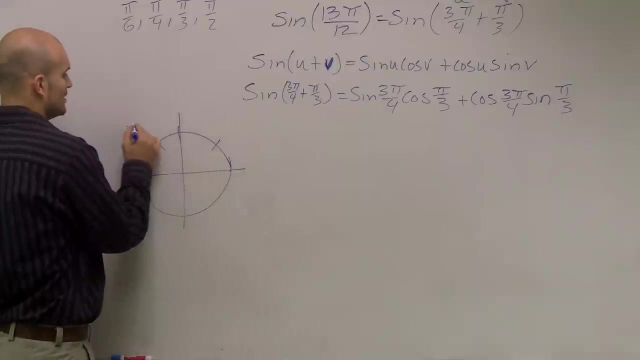 determine what these angles are. So I'll just draw a quick little unit circle here, And when I look at this unit circle, the sine of 3 pi over 4, 1 pi, 2 pi, 3 pi over 4 is right here. That angle is. 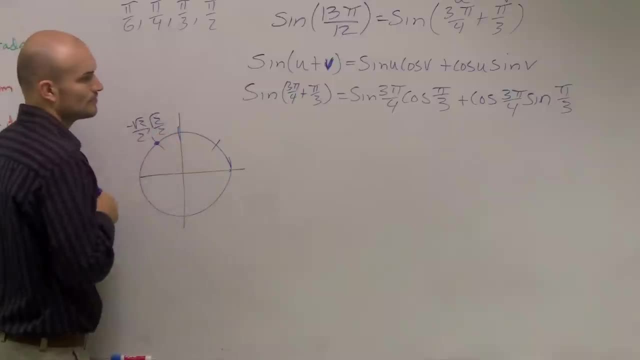 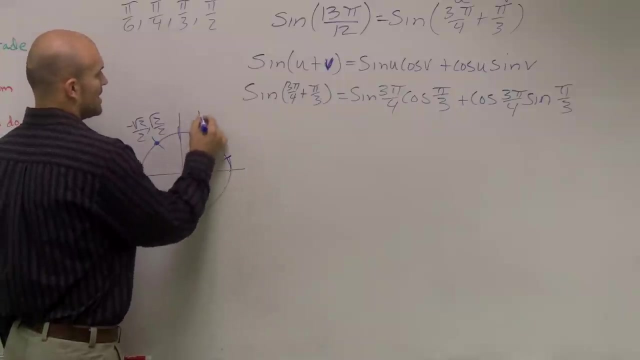 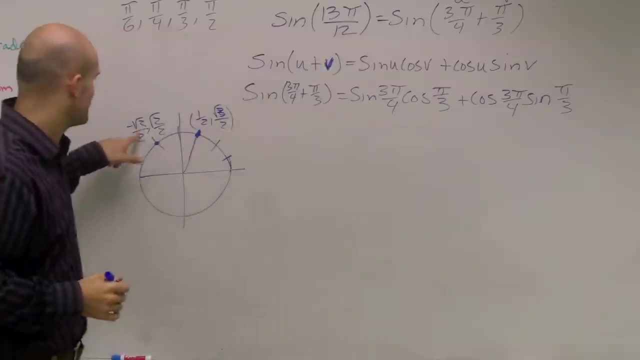 negative square root of 2 over 2, comma, radical 2 over 2.. And the cosine of pi over 3,, 2, pi over 2, is going to be this angle right here, And that point is 1 half radical, 3 over 2.. So the sine of 3, pi over 4,. 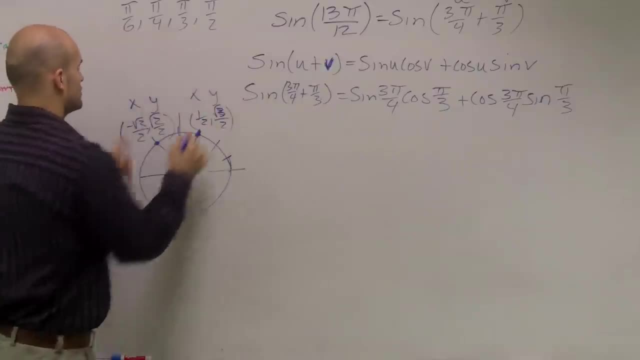 remember, is your y coordinate of your coordinate point. So the y coordinate of 3, pi over 4 is radical, 2 over 2.. The cosine of pi over 3 is my x coordinate, which is 1 half. The cosine of 3, pi over 4 is going to be: